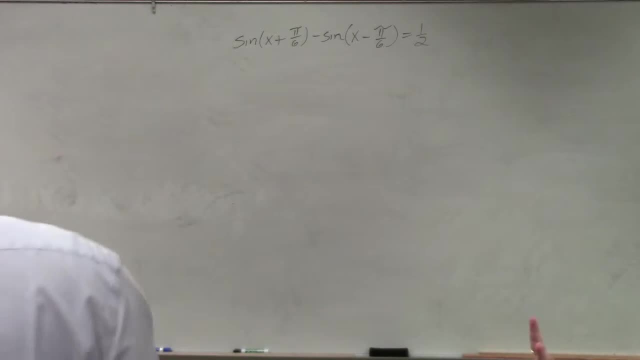 Do you guys see a sum and difference? Whenever you see a trigonometric function of the sum or difference, just apply the formula. OK, Just apply the formula So you guys can see here we have u and v And u and v. 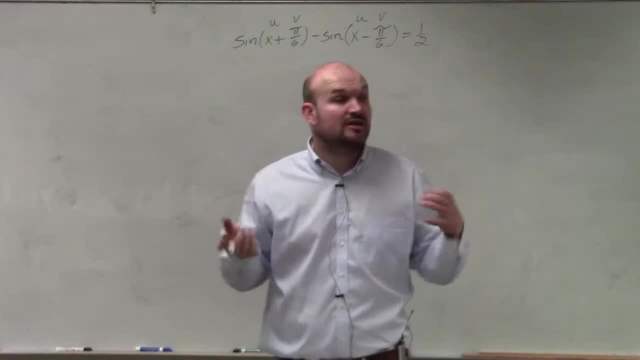 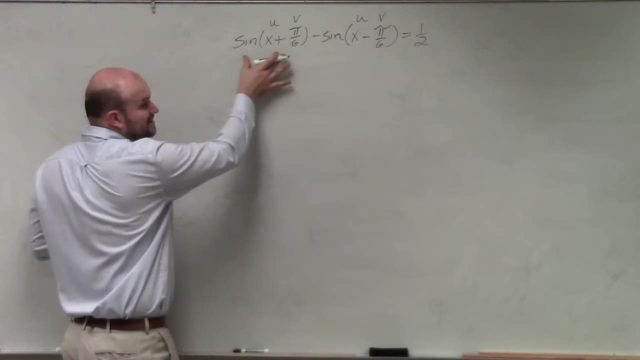 are different. The only difference between them is we have an addition and subtraction, which all that tells me is I need to use a different formula. Everybody agree with me. So first thing we're going to do is we're going to do this formula over here. 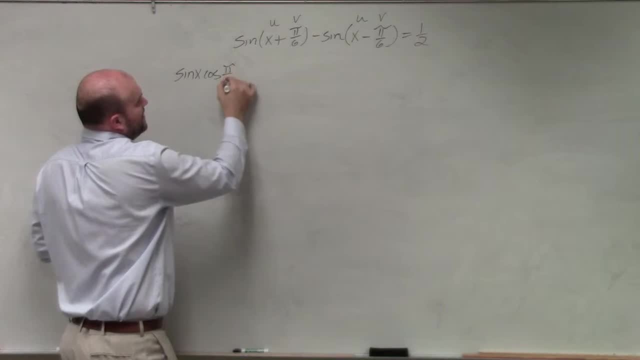 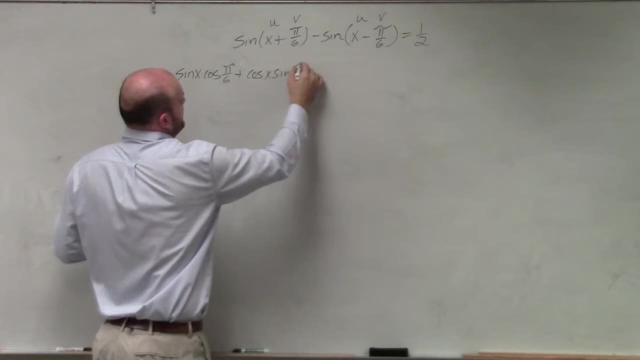 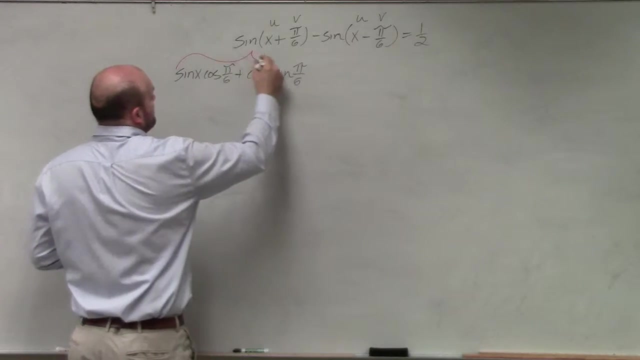 So this is going to be the sine of x, cosine of pi over 6, plus the sine of x, sine of pi over 6.. So what I just did is I did the sum and difference formula for that. OK. Now the next it's minus. 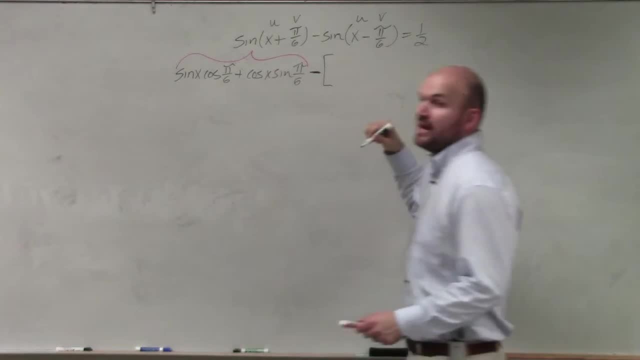 I got to make sure, though I'm subtracting the whole thing, So I'm going to put this in brackets. I'm going to include brackets, so I don't forget, I'm going to get something. Or don't forget, I'm subtracting that. 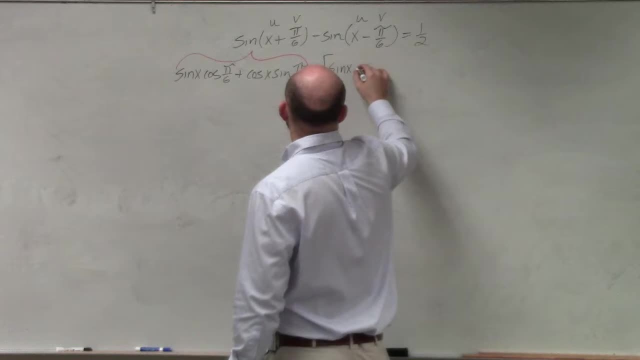 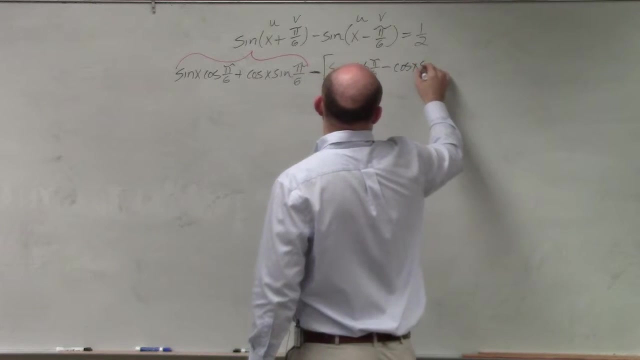 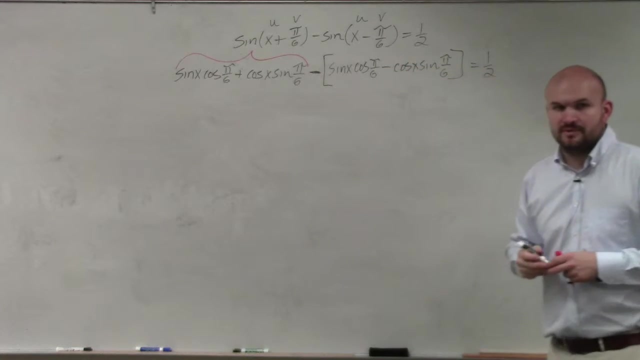 Now I'm going to do the sum and difference here, which would be sine of x, cosine of pi over 6, minus cosine of x, sine of pi over 6, and brackets equals 1 half. OK, The reason why I want to do brackets. 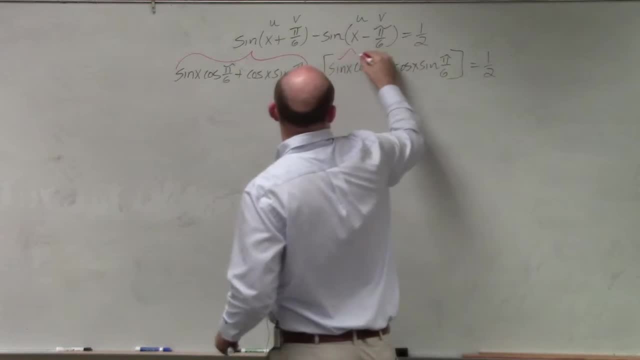 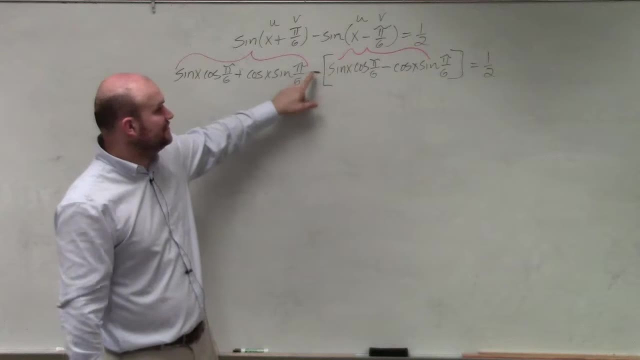 is because you're subtracting this whole thing. So OK, And what's important about that is, if I'm going to remove that bracket, what I need to do then is make sure I distribute this negative to both of these terms. Would you guys agree with me? 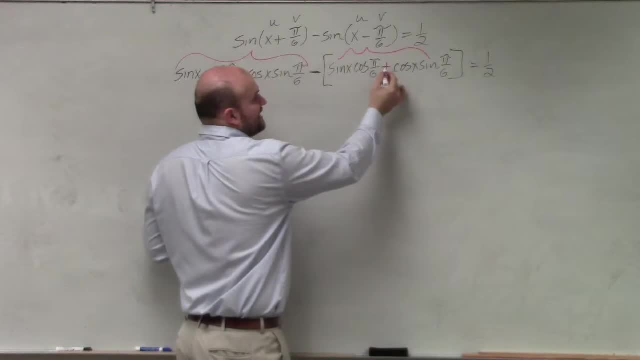 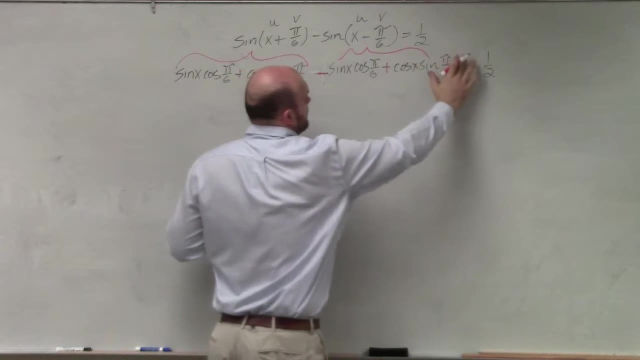 OK, so I can get rid of the brackets. I just need to make sure that that's positive and this is negative, And then I'll get rid of the brackets. Yes, All I did was apply distributive property with that negative. I distributed the negative to both of them. 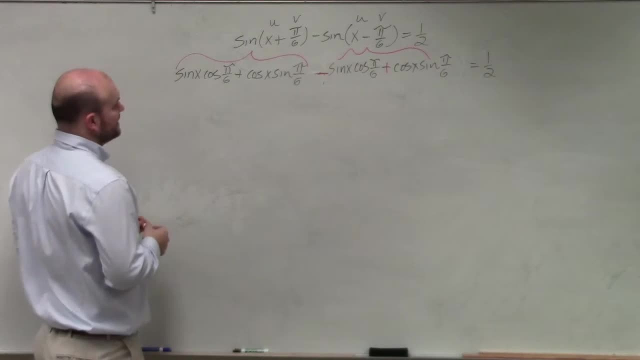 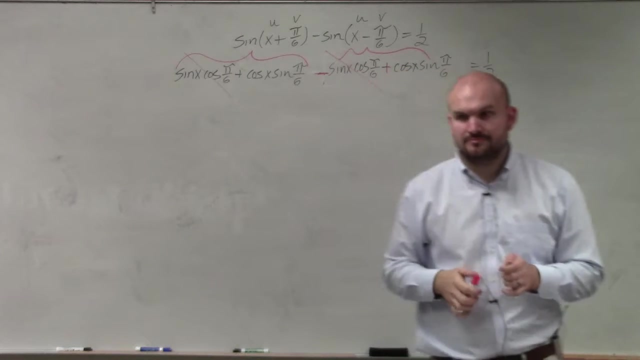 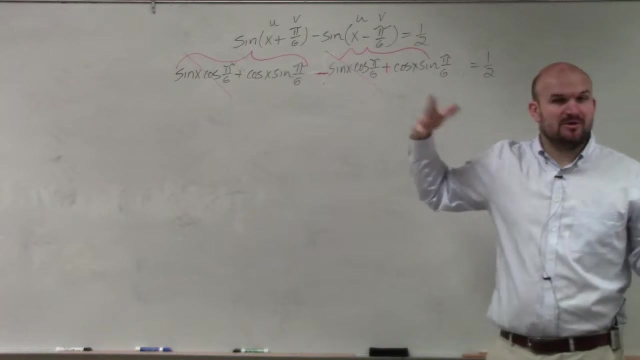 So that made that negative and that positive. Now, what I notice here Is these two terms are exactly the same, One's positive and one's negative, right, And then over here I have: these two terms are exactly the same. What's x plus x? 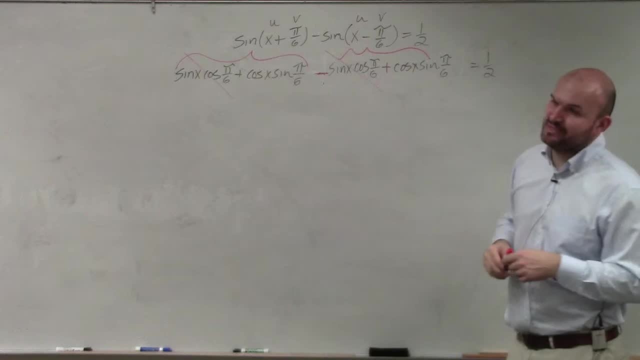 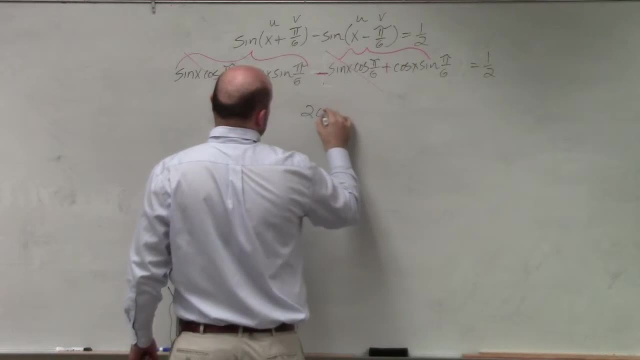 2x. So what do you think? cosine x sine of pi over 6 would be plus. cosine of x sine of pi over 6 would be 2, cosine of x sine of pi over 6.. So I do 2 cosine of x sine of pi over 6.. 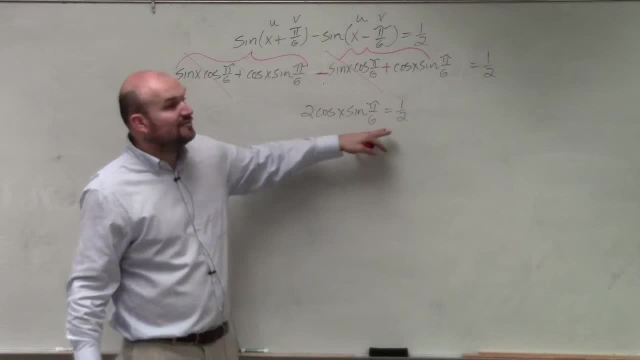 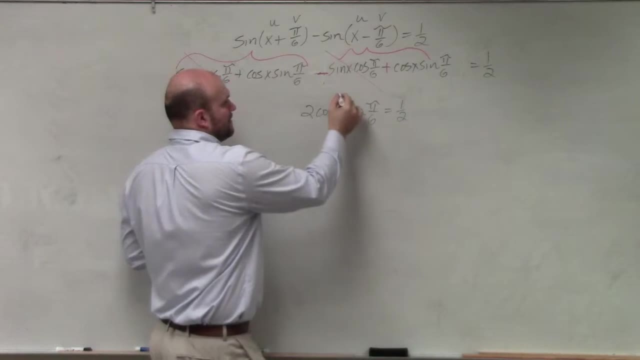 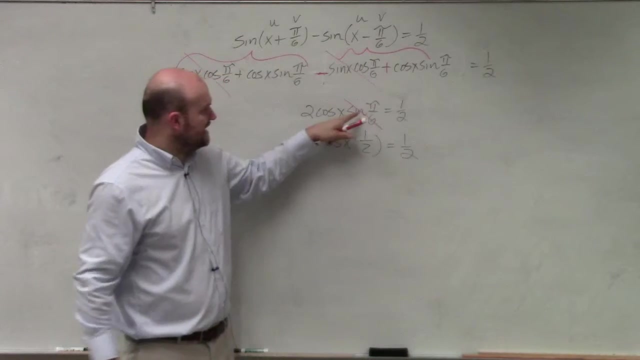 2 cosine of x, sine of pi over 6 equals 1 half. Now the sine of pi over 6 is going to be close 1 half. Yes, It doesn't. Sine of pi over 6 goes to 1 half. 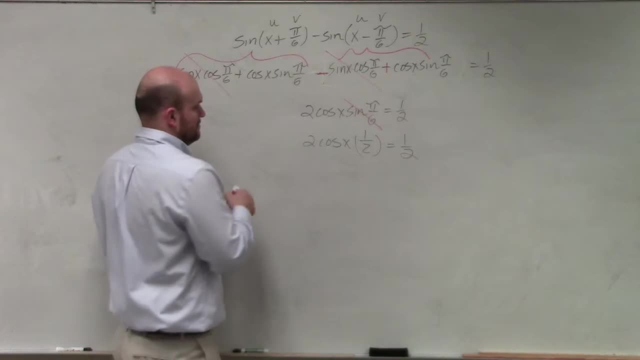 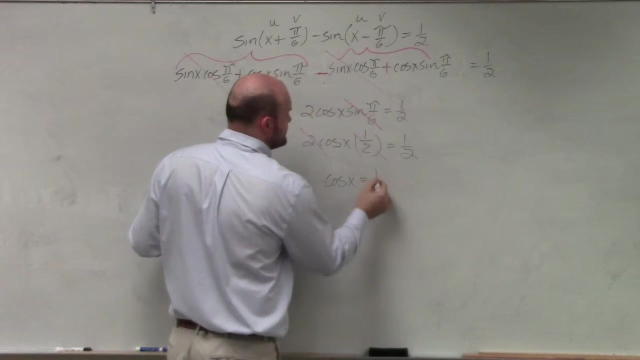 Look at the unit circle. What's 1 half times 2?? Now we have cosine of x equals 1 half. So what angles- And again I forgot to mention this- is finding all the angles between 0 and 2 pi. 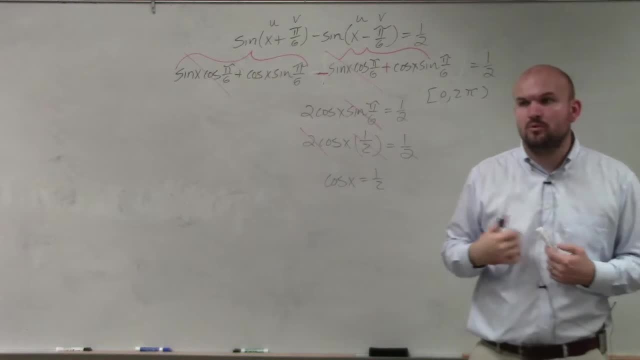 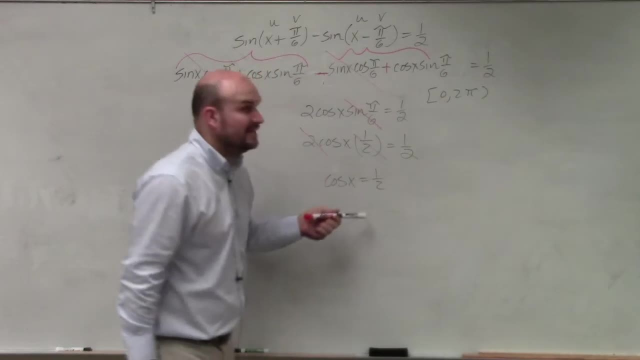 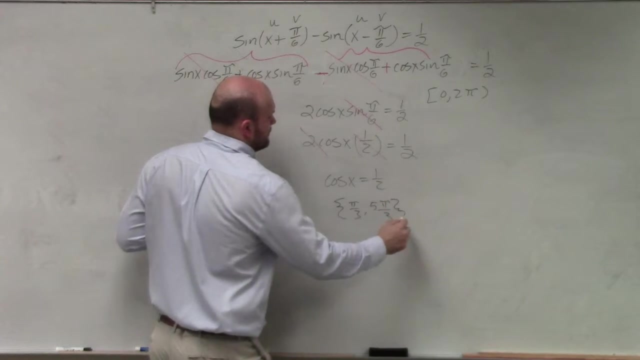 What are all the angles when cosine of x is equal to 1 half Pi over 3.. Is that the only one? And Yes, So why isn't it 2 sine pi over 6?? Why is it what Not 2 pi sine over 6.? 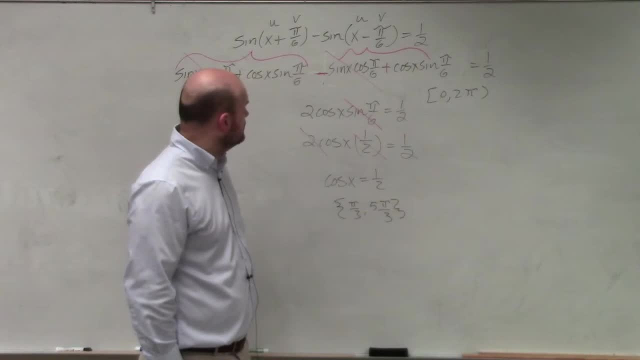 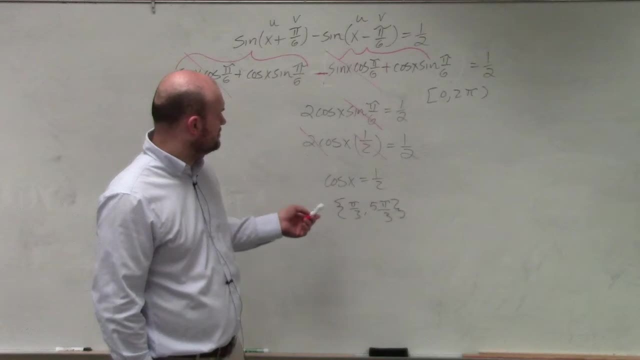 I mean no, no, no, no, no. 2 sine pi over 6. Because it's 2 sine pi over 6. 2 sine pi over 6. 2 sine pi over 6. Right here. 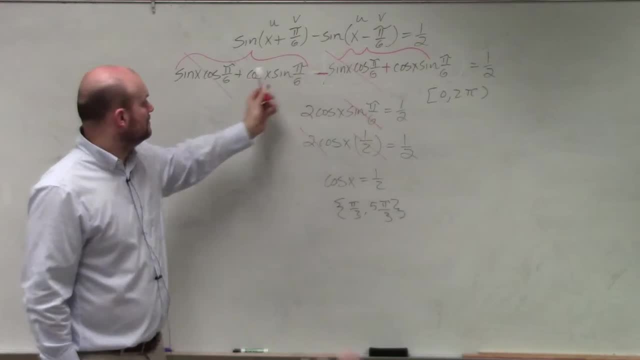 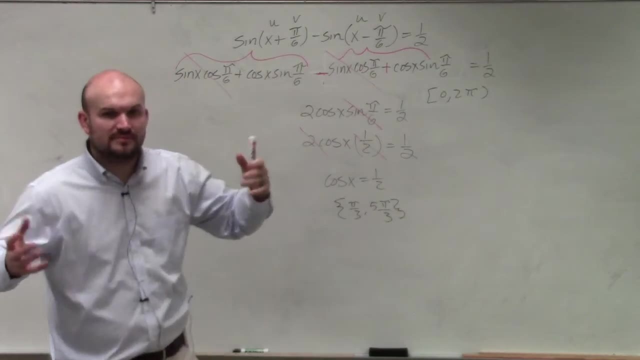 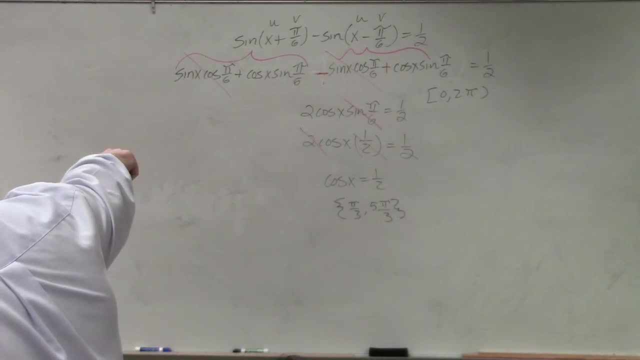 Yeah, but that's positive and that's negative. Yeah, so it's 2 cosine, It's one term. Think of them like as an x. Yes, Why did you get rid of sine? Well, because sine of pi over 6, what does that equal to? 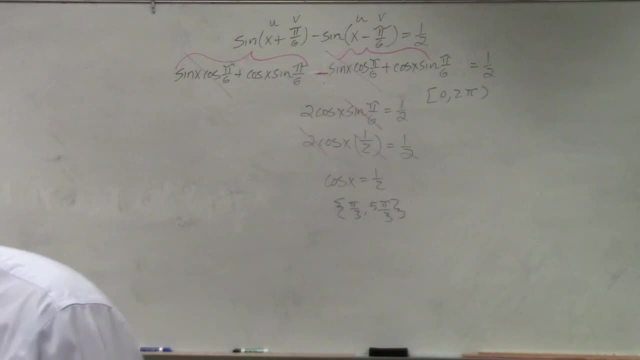 1 half Sine of pi over 6, that is 1 half. So I didn't get rid of that. I mean, I did get rid of it, but I just evaluated.